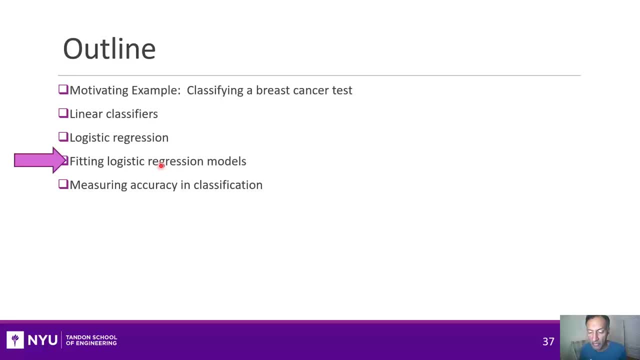 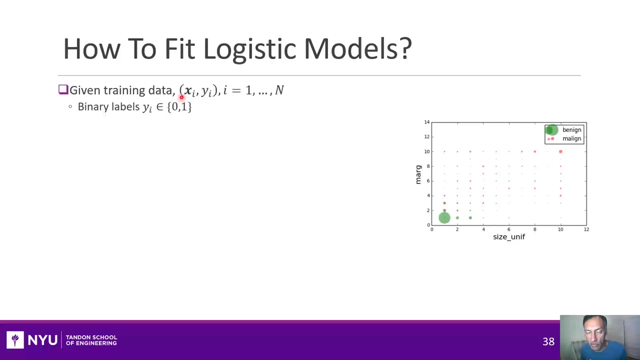 Okay, so in this section we're going to look at a little bit of the mathematics about how to fit logistic regression models. So to set that problem up, let's say we have some data and let's just, for the time being, look at the binary classification problem. 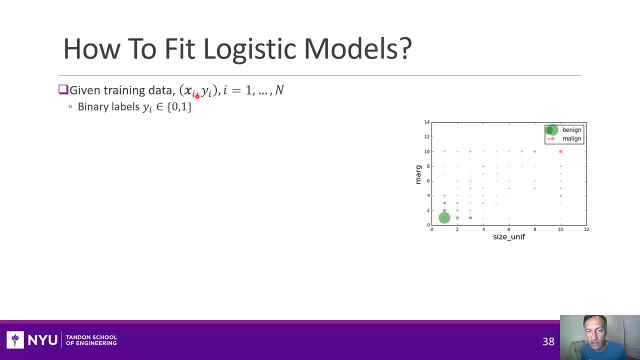 So we have n data samples. each has a feature vector xi and a binary label. So for example, in the breast cancer case we would that feature vector would have two features, the size and the margin, and each sample would have some label. In this case I've drawn it with a red or a green dot. 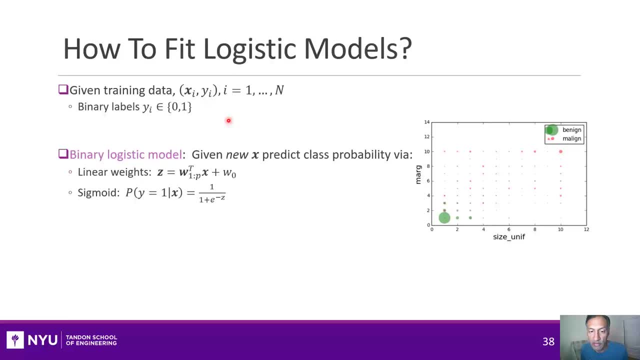 Now, what we were talking about in the previous section was that we wanted to fit a logistic model, and a logistic model just means that if I have a new sample x, I'm going to predict its probability of being in a class by doing two things. 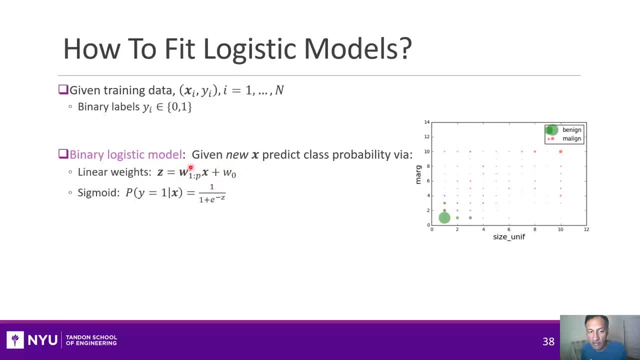 I take a linear combination of the features and it gives a scalar z and then from that z I compute its probability. Now, when you look at that model, it has some unknown parameters which are the vector of coefficients w. So you could. 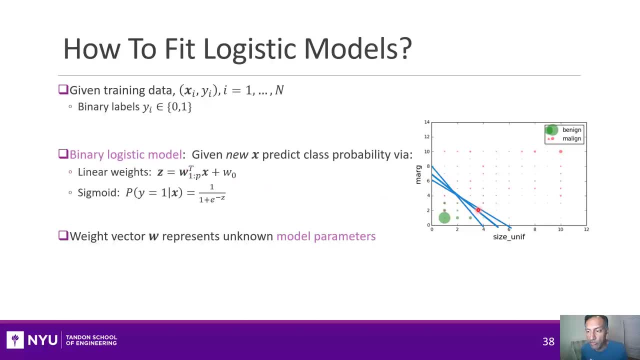 graphically represent that w as shown here. Now, when you see this, you can see that there are a lot of different possible w's that seem reasonable for partitioning these green circles from the red ones, And the question is: how do we select the correct w? 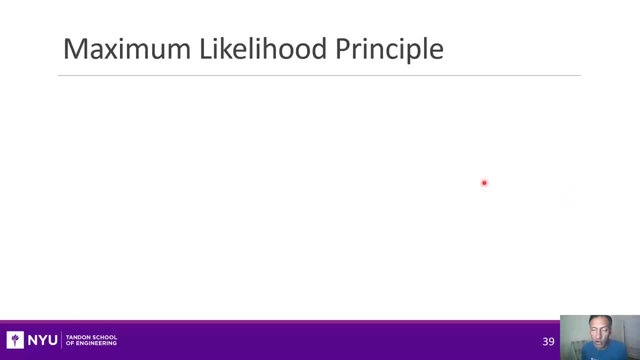 So the key concept is what we call the maximum likelihood principle. So you would have seen this definitely if you took the probability class, and certainly in the detection and estimation class. But even if you have never heard of it, it's a pretty simple concept, at least in concept, in theory. I'm going to walk you through it. 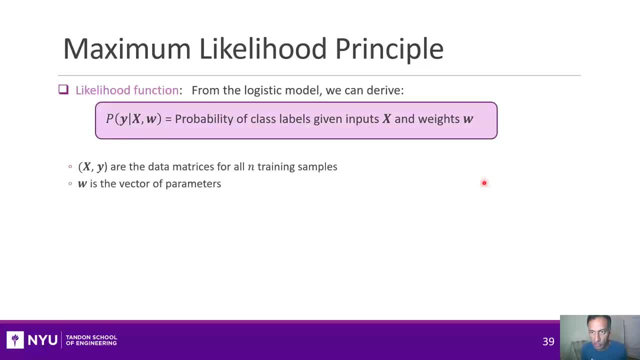 So the idea of the maximum likelihood principle- and it applies very generally- it starts off with something called the likelihood function And it's just this mathematical conditional probability. So you see, it has three variables in it. There's our data x, our output y and our parameters w. 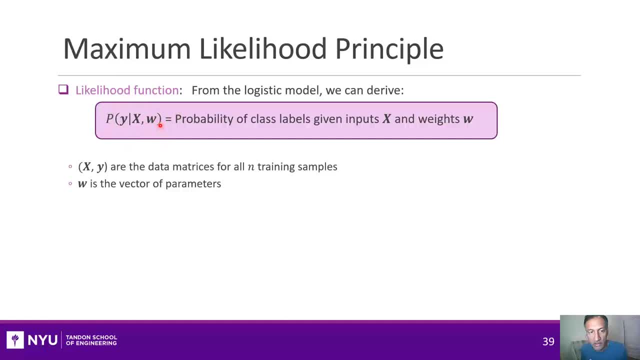 And all this mathematical expression says is that if I gave you the inputs x and the parameters w, what is the conditional probability that I would have seen y? Alright, and this is over all the data. Now, why would I be interested in such a function? 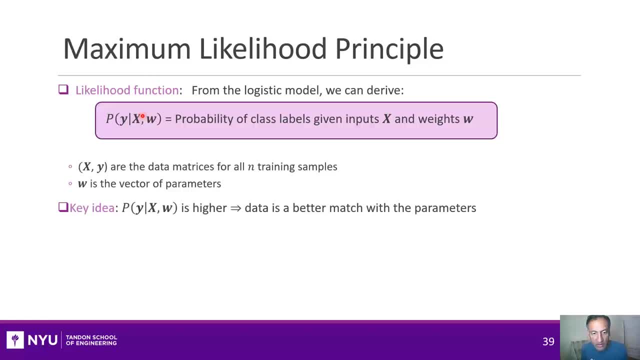 I'll show you how to compute it In a moment. The key idea is that this quantity, this conditional probability, the likelihood, should be higher whenever the data is a better match with the parameters, Because it says that well, given this input and 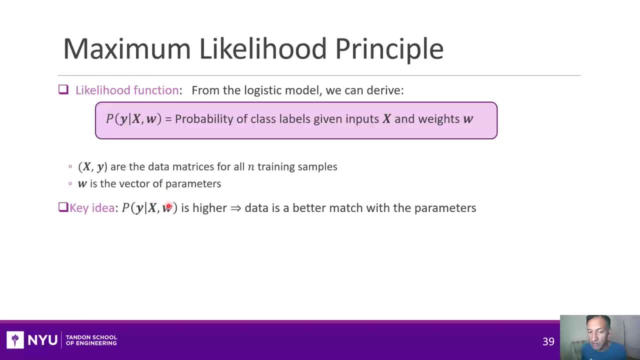 given this w that some candidate parameters. this is high, It means that that w, that y that I did see, was very likely to have occurred from this model. On the other hand, if it's low, it means that it's not really consistent with that parameter. 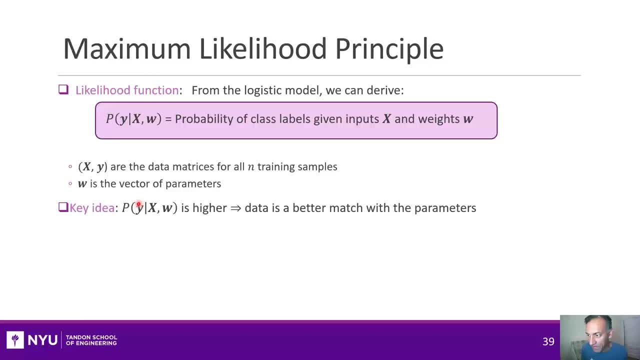 Now you probably already got the main idea. The key idea in maximum likelihood is that I just pick the w, the parameters, to maximize that conditional probability or maximize the likelihood. That makes very good intuitive sense. If you take the detection and estimation class, you will also learn how to do that. 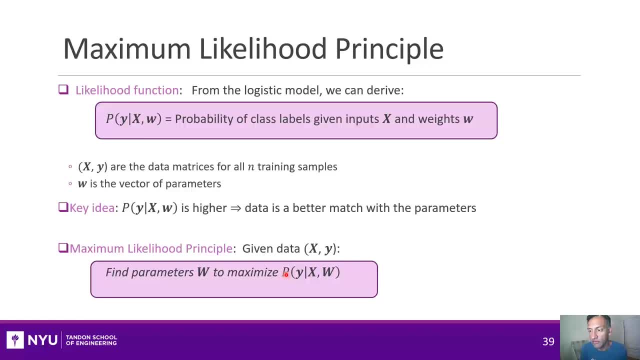 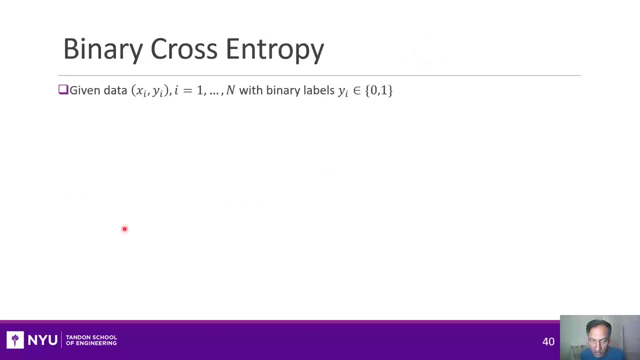 So I'm going to show you how to do that. In turn, it has very good statistical properties, But we don't need that. if you can just trust the idea that this is a generally good principle to develop any estimator. With that in mind, I'm going to show you how to compute the likelihood for the binary classification problem. 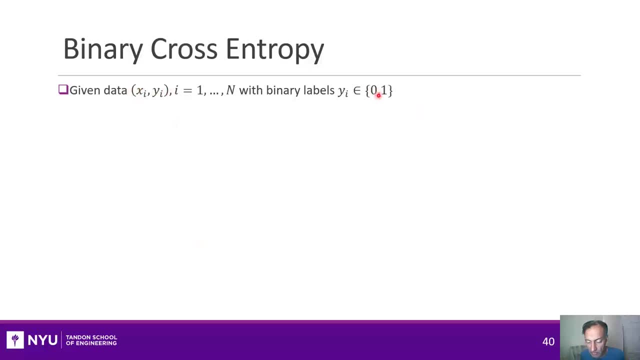 So again, imagine we have n samples with binary labels. The key idea is this result, That is, that if you do maximum likelihood estimation for the logistic model, it's equivalent to minimizing this function, And this function here is called the binary cross entropy. 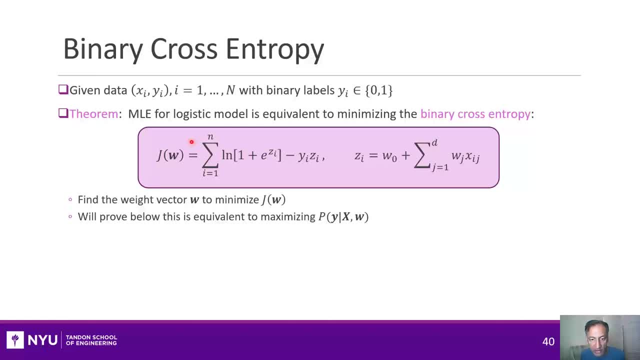 I'm going to graphically show you that in a second. Let me just- and I'm going to prove this also below- But let me just show you a few things. The first and most important thing is that this function just gives you a simple procedure to write the maximum likelihood estimation problem. 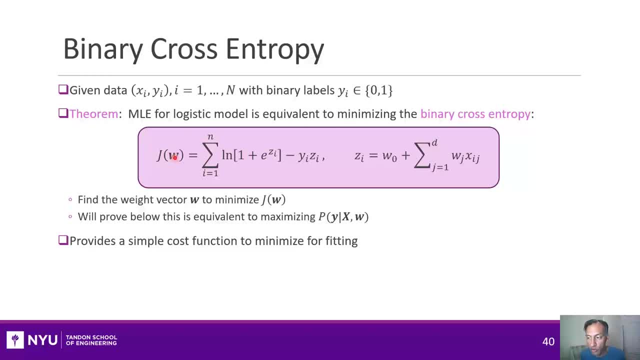 as minimizing some function. If you recall, when we were looking at the linear regression, we were just minimizing that squared error. Here we're just minimizing a different function which happens to have these log terms. Now, one thing about that function. 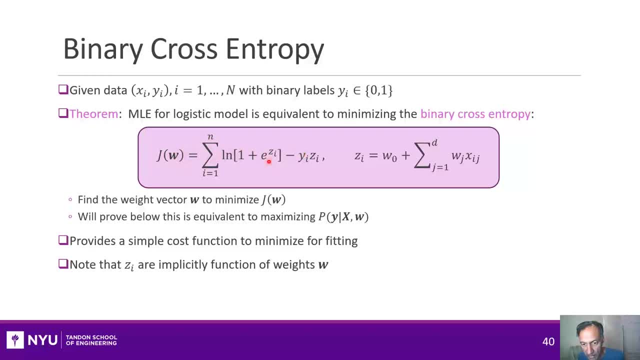 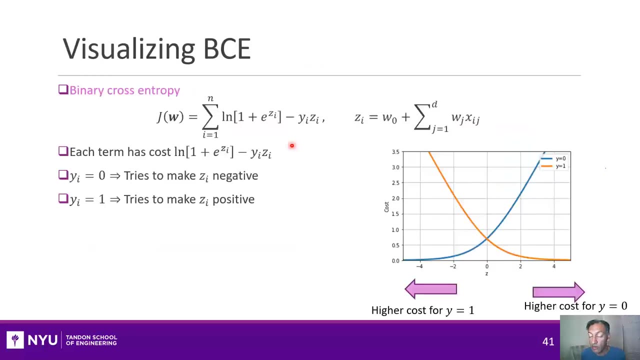 You see here that the function on the right-hand side depends on these z? i's, But the z i's depend on the w's through this second equation, So the z i's are kind of implicitly depending on the w's. Now let me try to, before proving that this is indeed the same as doing the maximum likelihood, 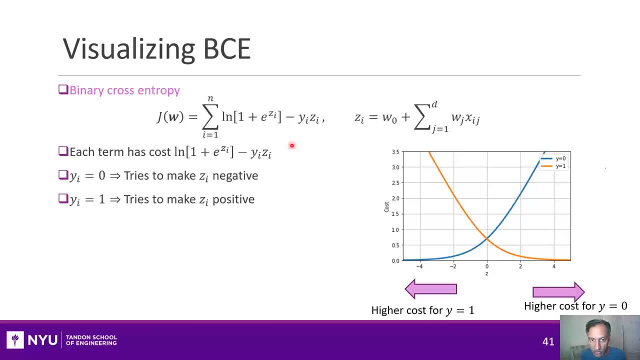 let me show you some graphical properties about this function. So here's our binary cross entropy function And you can see it's a sum of terms And each term is like this: This function is a function of two things: the z? i and the y i. 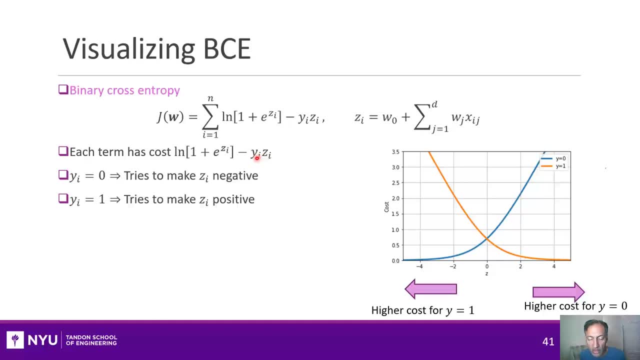 The y i can be either 0 and 1.. So let's take a look at the curve. when y i is 0. And that's shown as a function of z. It's shown here as blue. So what this means is that if the sample is 0,. 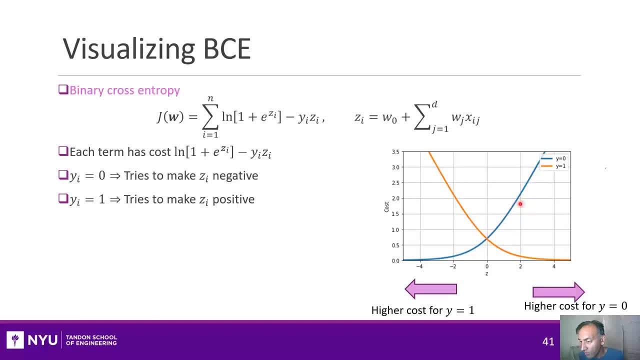 it will have a higher cost as z is larger. Now that means when you're trying to minimize the function, it will try to make z less than 0. In fact, it will try to make it as negative as possible. On the other hand, if the sample is positive, 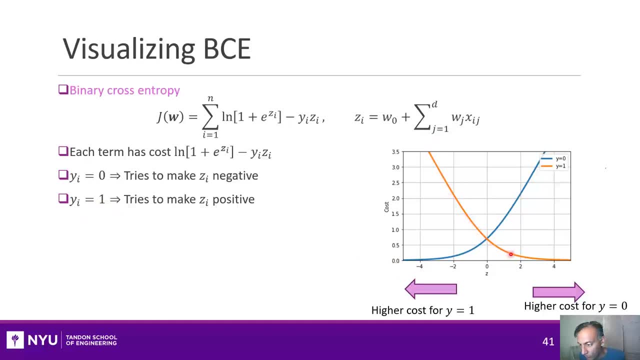 that's y, i is 1, the function looks like this orange curve. If you try to minimize that, it will try to make z as high as possible. So it's going to try to make z large. on the negative samples, sorry, the positive samples. 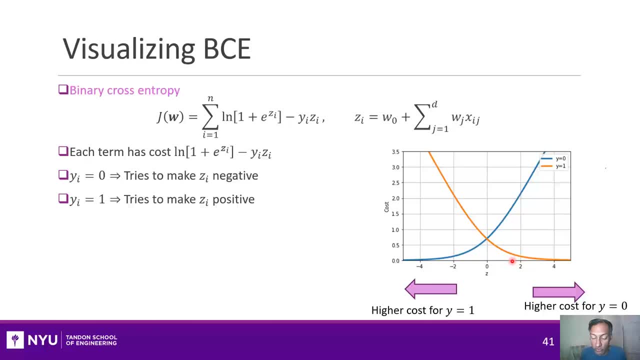 And z to be large negative value on the negative samples. Now if you go back and you think of what happened in the case of a hard decision classifier, the classifier would always select y hat to be 1 when z is positive and y hat to be 1 when z is negative. 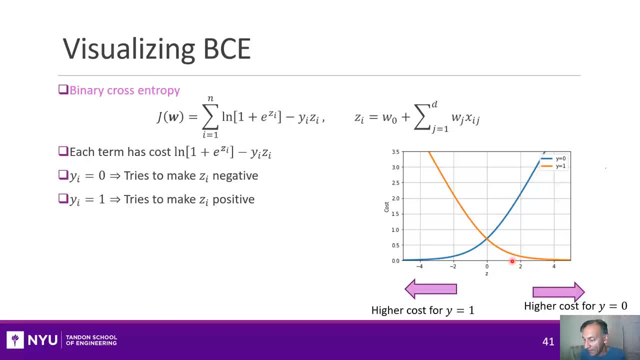 So this is trying to make it not have any errors, But it allows you to make mistakes. In other words, even for the negative samples, you're allowed to make z positive, Or for the positive samples, you're allowed to make z negative. 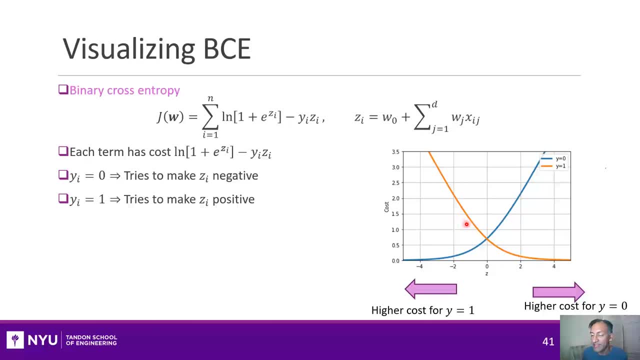 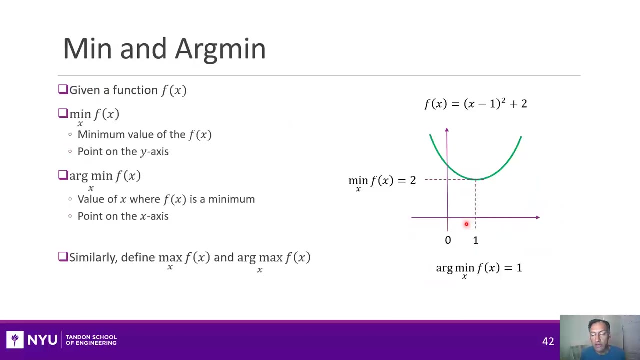 but you just do it at a cost, Because this is the idea that the logistic model doesn't expect that the classifier is ever going to exactly produce 0 training error on any data set. Now. now I want to turn to just proving this binary cross entropy formula. 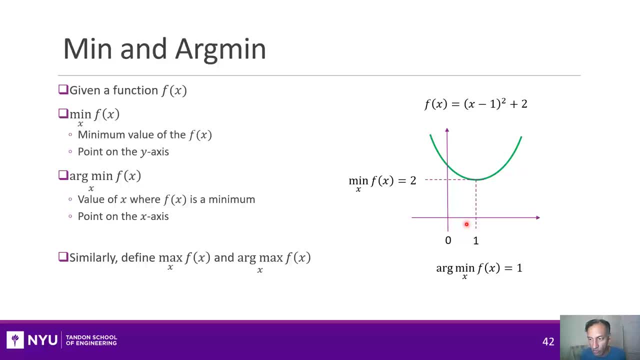 So we just need to do a little bit of math. It's actually pretty straightforward. It's more just about notation. So the first thing we need to look at is something called the min and the argument. So if you just go back to calculus, 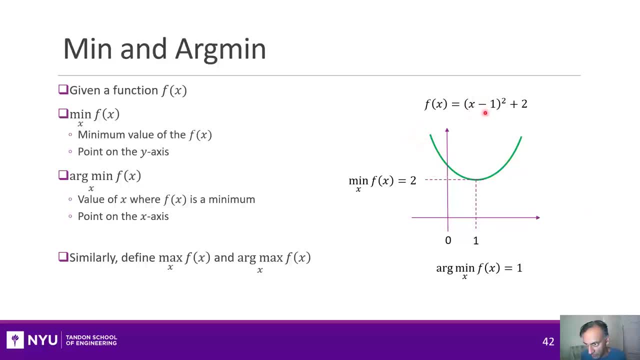 and I draw a function of x. any function like this quadratic. we all know its min is the smallest value on the y-axis. So that would happen in this parabola. The smallest value would be 2.. So if a mathematician writes min over x, of f, of x, 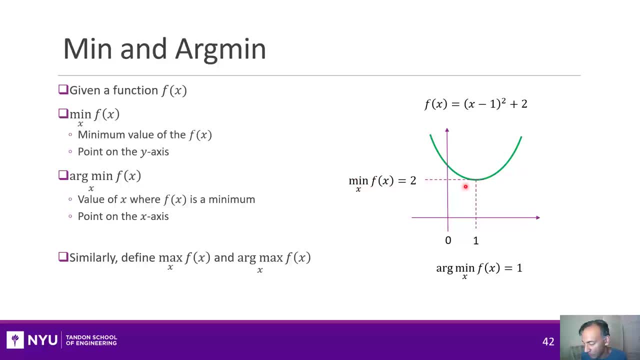 they're talking about the value on the y-axis. So this is probably what you saw in calculus. What you might not have seen in calculus, which is an equally easy idea, is the term argmin, And argmin just means the value on the x-axis. 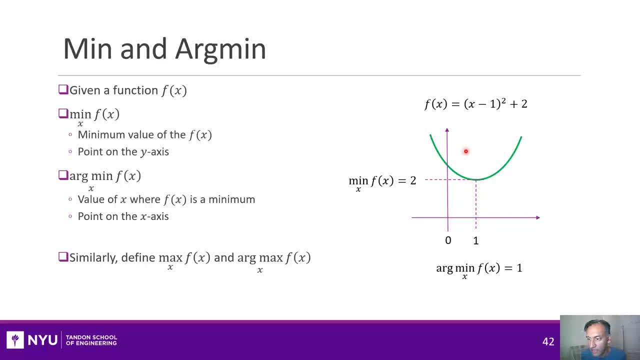 that produces the minimum value. So in this case, the function achieves its minimum when x is 1.. So we say: argmin of x, of f, of x equals 1.. Just a mathematical notation for a concept that you already understand. So now, if you see argmin, don't be scared. 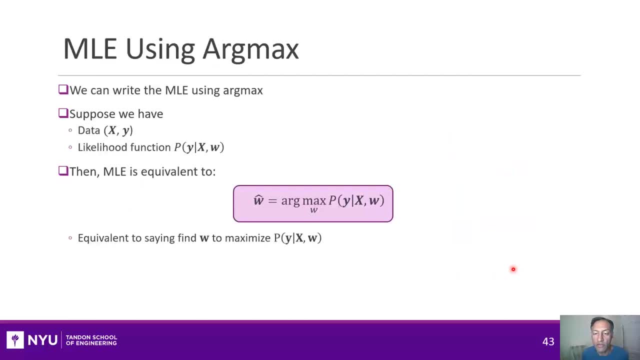 That's all it means Now. the use of this for us is that we can say that maximum likelihood is just. we want to find the w that maximizes this likelihood or this conditional probability. Or using my mathematical notation, I want to say I want to find w hat. 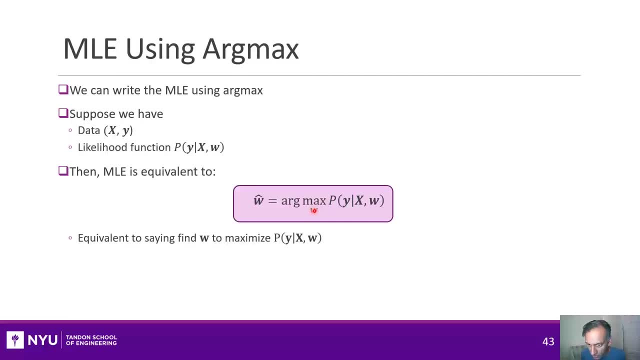 is the argmax over w of p, of y, given x and w. So that's all it means. So it looks really intimidating, but it's just this. This thing is not that hard, It's just the conditional probability of seeing the labels. 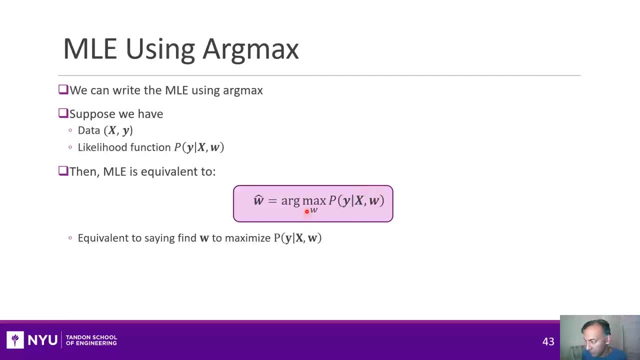 given the parameters in the input, and then I'm going to maximize that. So it's just notation, to express an idea which you probably understand already. It's just putting it into mathematical notation. Okay, Now we're going to go about proving this binary cross entropy formula. 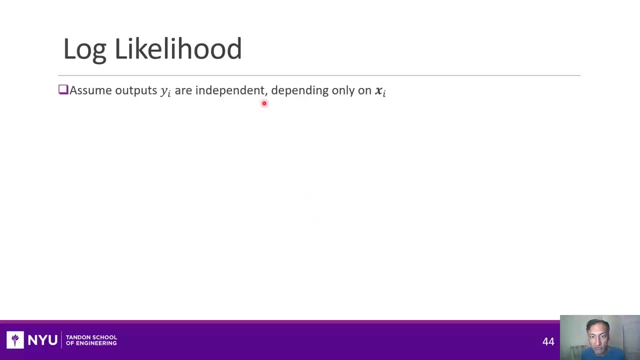 It's a couple of steps, but none of them are that hard. The first is that you make an assumption that in this model the output on each sample are independent and they depend only on xi. Now, if you remember back from probability, 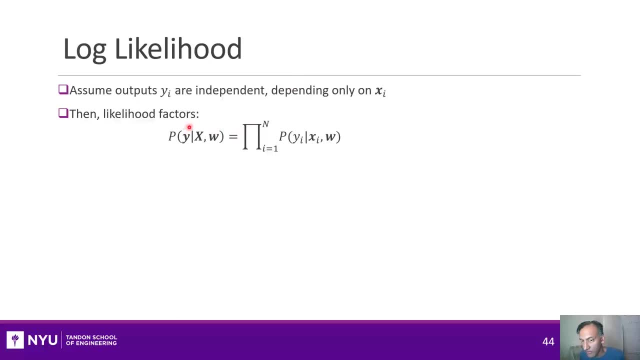 if you have a bunch of independent, random variables, they factor. So if I have the vector of all the samples, that conditional probability, the probability, that joint probability, will just be a product of the probabilities on each sample. Okay, So now we only have to look at one sample at a time. 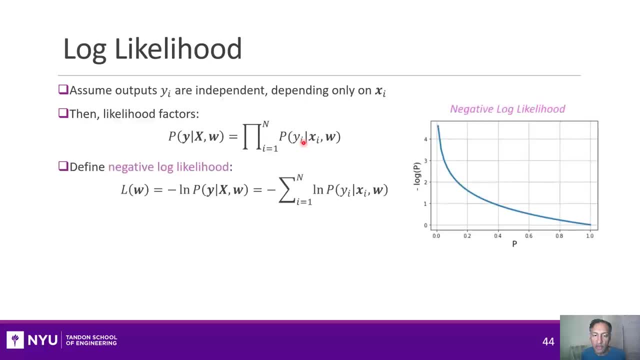 Now the next thing to do is to introduce something called the log likelihood. Instead of trying to maximize this, we're going to look at the negative log of this, So we're going to call that L, And this is just the negative log of this probability. 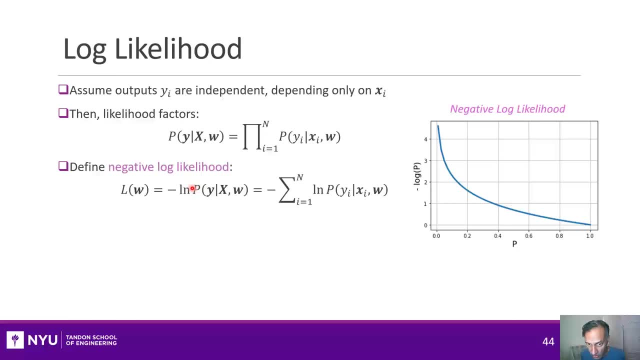 And the reason why we want to look at the negative log is because, if you remember, log of a product is the sum of the logs, So it converts products to sums. And that's all I've done in this next step. Now the key idea. 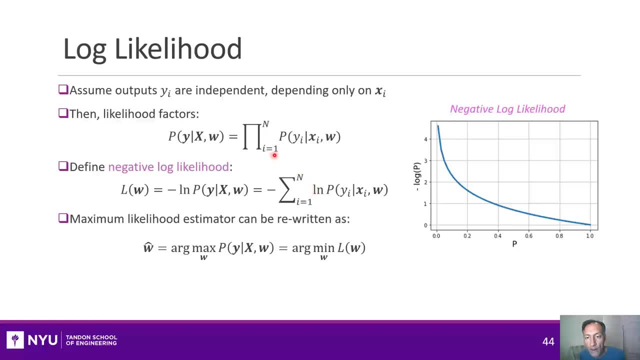 then is that if you want to maximize this probability, it's the same as minimizing the negative log. Why is that? Because here on the right I've drawn this log likelihood, So it takes this probability p and converts it to negative log of p. 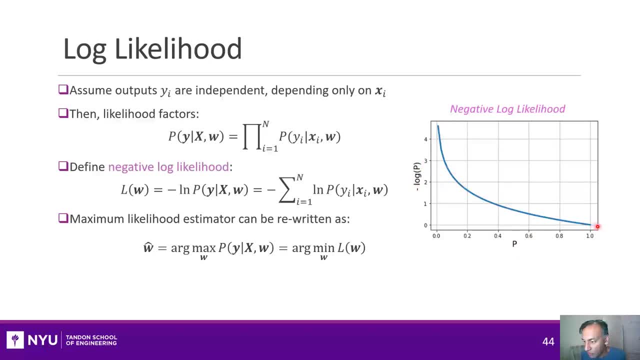 And you can see here that it monotonically decreases. So that means that if I want to make this p as large as possible, it's the same as making the negative log of p as small as possible. Alright, So all I've done here. 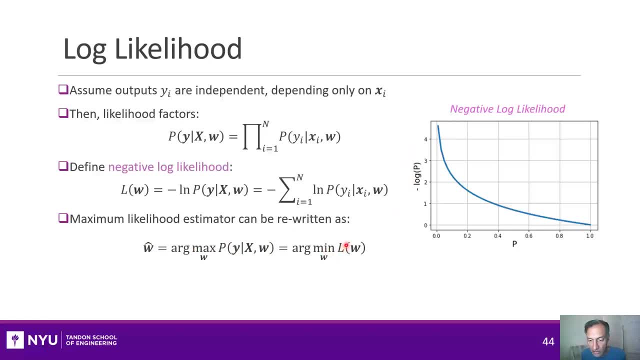 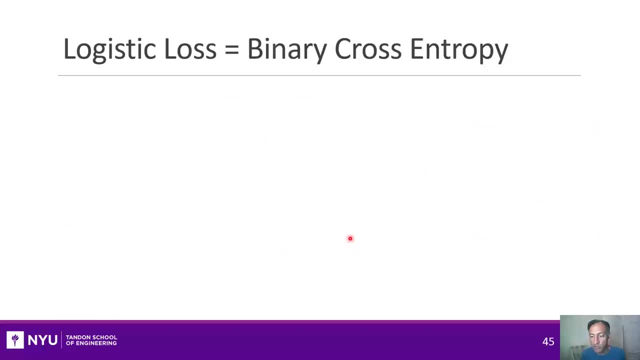 is just done this, So we just need to minimize this negative log likelihood And now, with that bit of preamble, we can prove our result: That we want to minimize this binary cross entropy. It's just this, Okay, so our negative log likelihood: 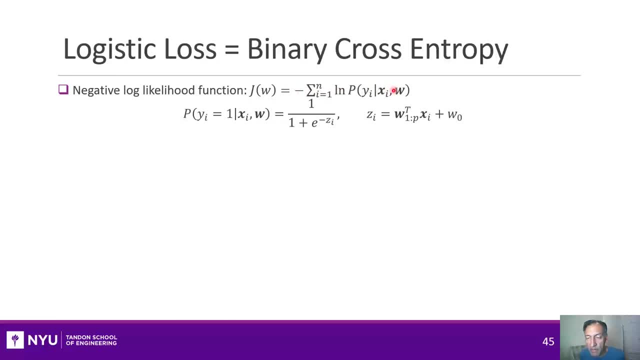 will just be this, But remember that in the binary cross, in the binary logistic model, the probability that a sample is 1 is this: 1 over 1, plus e to the minus z, i Alright, And therefore the probability that it's 0. 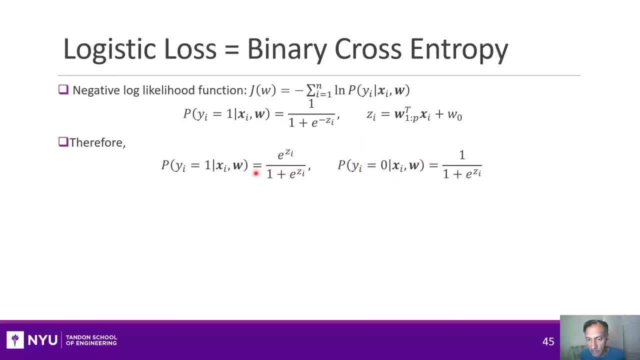 is 1 minus this, And so you can write it like this, Just doing a little bit of mathematical rearrangement, Not too hard, And therefore you could write this little trick Right. You say that the log of this. well, 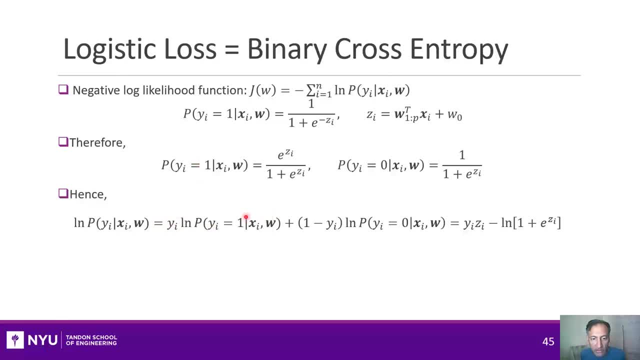 when y i is 1, it's this value. Alright. When y i is 1, it's well the log of this. And when y i is 0, it's the log of this. And when you substitute these expressions in here. 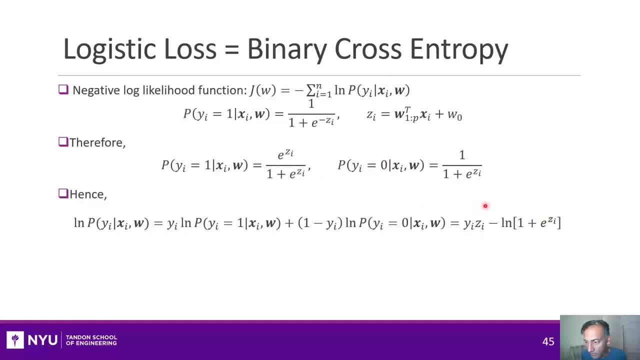 and do a little bit of math, which I'm not going to waste your time- you get this expression here, Alright, And then if I want to take the negative log likelihood of this, I just take the negative, the sum of the negative values of this. 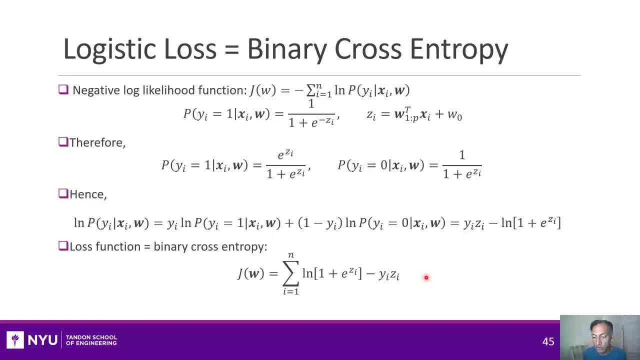 And that is this function here Which is, you know, the binary cross entropy. So I've just done a little bit of math and algebra to get you that function that we saw earlier. Now all of this extends to the multiclass. 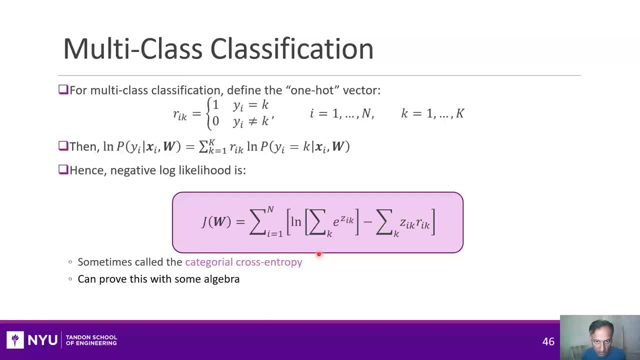 I won't walk through all the details, but it's pretty similar. The only weird thing is that you have to to write the function. you need to find this kind of one-hot coded vector And you say r i k is one, when the label is the k-th. 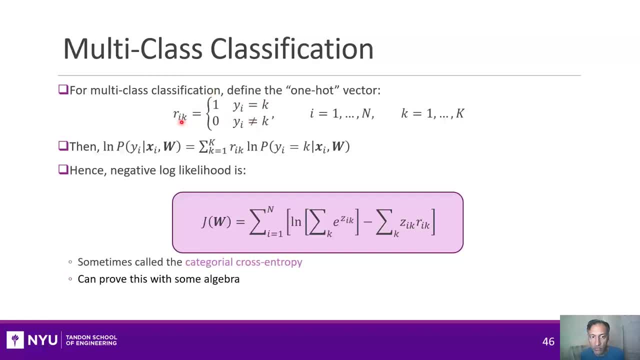 class and zero otherwise. So for every i r, i k is one for exactly one class, And then we're going to just say that the log of that probability is going to be the sum over these k's of this Same trick that we pulled. 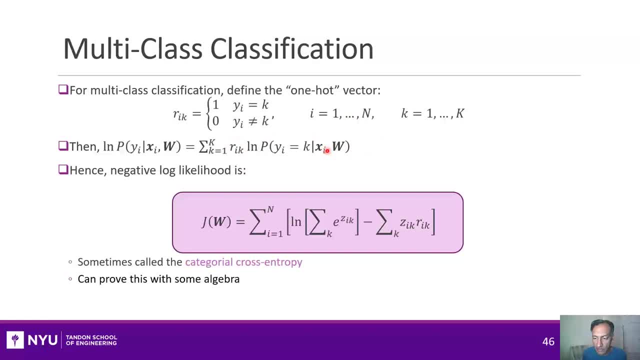 And then after this and a little bit of math- not too much, I think it might be on your homework- you get this function here And it's pretty similar in form in that there's a log of a sum of exponentials and then minus some other sum here. 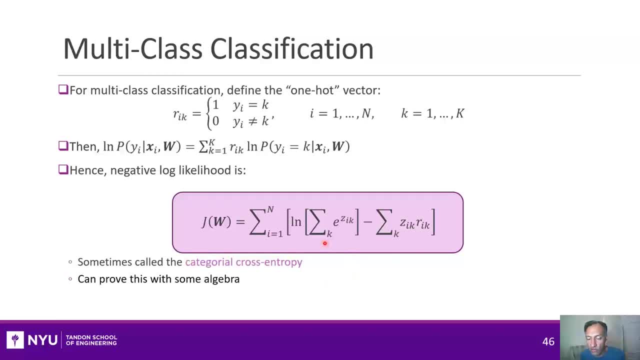 And this is sometimes called the categorical cross entropy Right. So for binary classification we have the binary cross entropy And for multiclass classification we have categorical cross entropy, And I don't want to waste time going through this derivation, just so you understand. 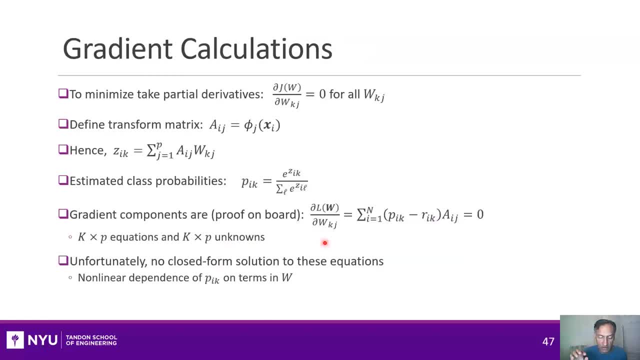 these two functions Now. now I have a function that I want to minimize, So how do we minimize it? Well, a trick we learned before in when we were looking at logistic- sorry, when we were looking at linear regression- is we had our function. 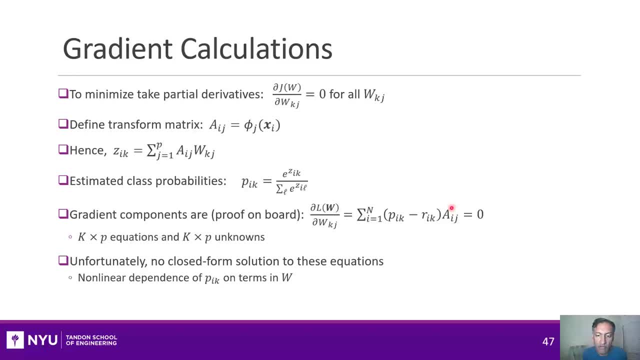 and we took the derivatives and set it equal to zero. So I've given some math here, alright, which I don't want to bother going into. You could do that here. You could take the derivatives, you could set them equal to zero. 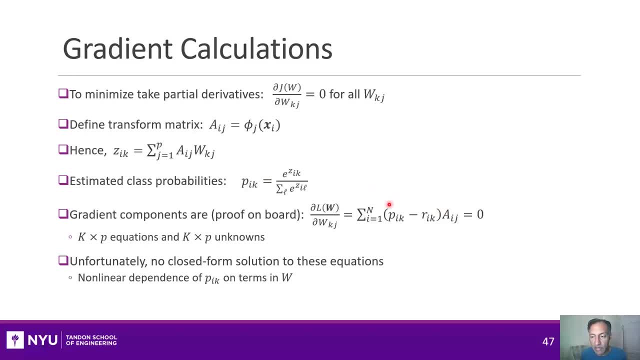 and you get some expression. But the problem is this expression gives you, it gives you p equations and p unknowns, which is great, but they're non-linear equations. There's no analytic way to solve them, If you recall what happened in linear regression. 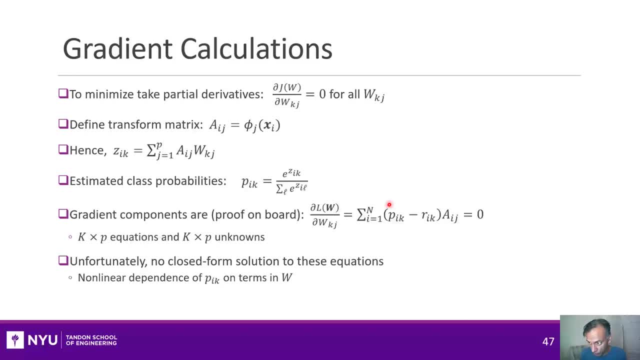 you could actually just, in closed form, write what the solution to those equations were, But we can't do that in this case. So how do we go about it at this point? Alright, we have to step back and think in general. 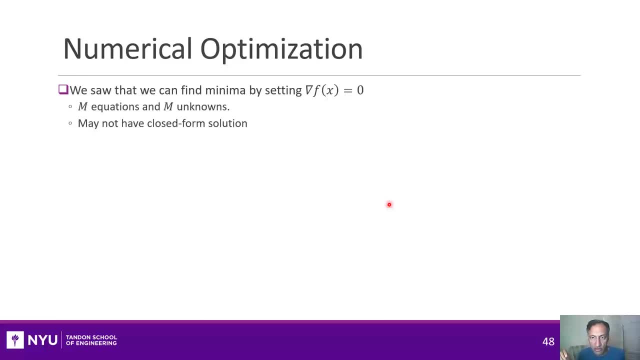 about how we try to minimize functions. So if I have any function of some variables like x, and if they're m, x, if x is a vector with m coefficients, I would take its derivative or its gradient and set it equal to zero. 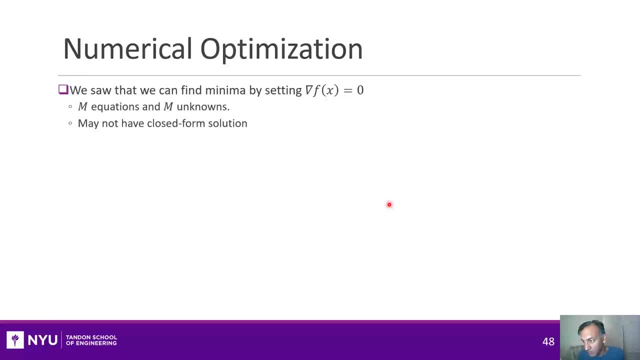 And I get m equations and m unknowns, But sometimes you can't solve that, like we've seen. Instead, what you have to do in these cases is do what's called a numerical method, And a numerical method is a computer algorithm. 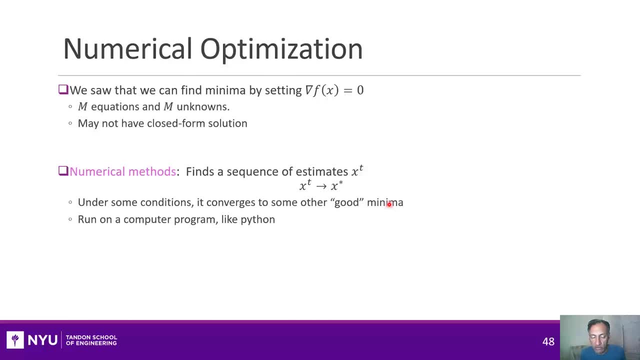 that starts at some guess for x and tries to get a sequence of points x that eventually converge to a good minimum, And then you run this program on your computer Turned out. we're going to cover this- how to do this- in detail. 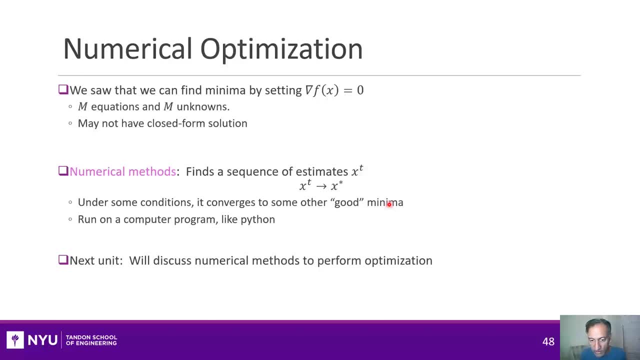 or not. I wouldn't say in detail but touch on it in the next unit. But for today's lecture I'm just going to use a built-in Python routine. So I'm just going to run it on the computer and it will solve this for us. 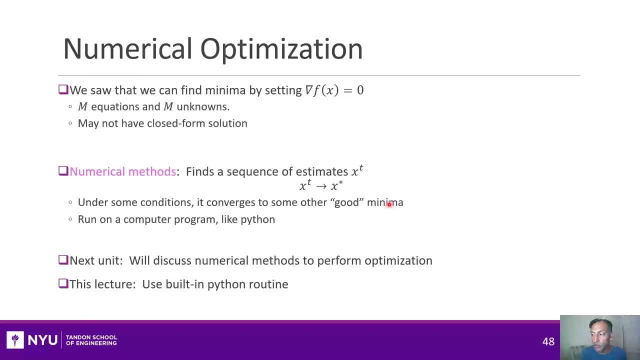 And in next unit we'll kind of open up the hood and see how that works. But for now just understand that there is a function we're trying to minimize and there's a computer algorithm that finds that minimum for us using some numerical method. 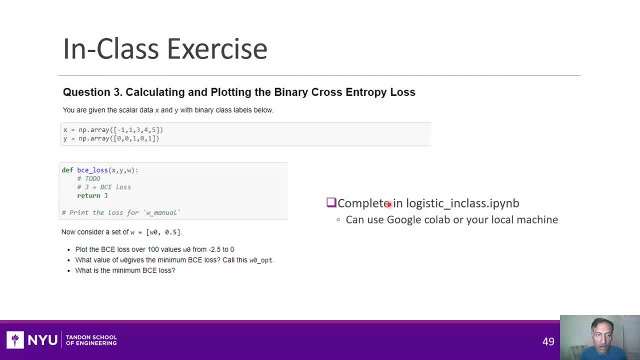 Alright, With that in mind, before we go on, before you go on, go to the in-class notebook and I've put a very simple exercise where I've given you just some very simple 1D data and I want you to plot that binary cross entropy loss function. 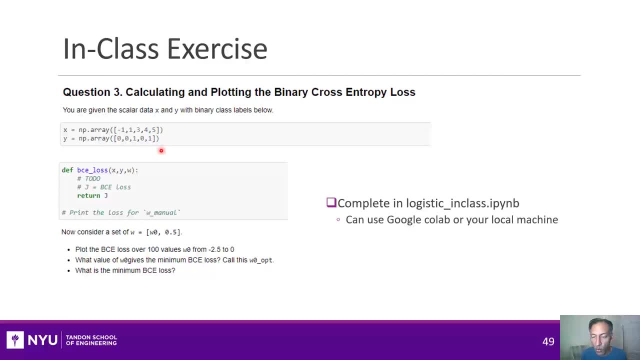 as a function of the parameters of this in this simple 1D model, just to give you a little bit of visual sense of that loss function. And once you do that, you can proceed on to our next section.